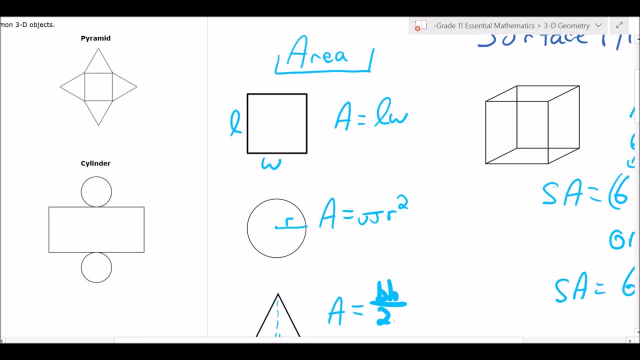 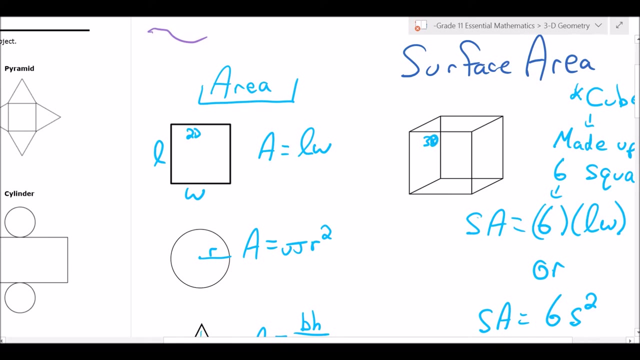 area. Now area works with two-dimensional objects. So a two-dimensional object is something that is flat like a piece of paper. Now we're going to work with three-dimensional objects, So this guy here would be a two-dimensional object. This would be an example of a three-dimensional object. 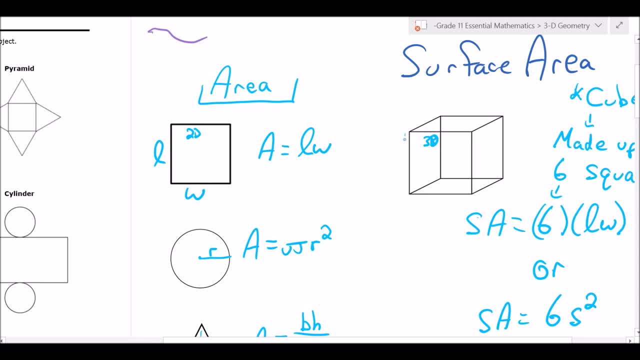 A three-dimensional object obviously has one more dimension. So we might have one dimension here, up and down: length, width, and now we'll have depth. So an example of a three-dimensional object would be a cup, would be a box, would be anything that has a third. 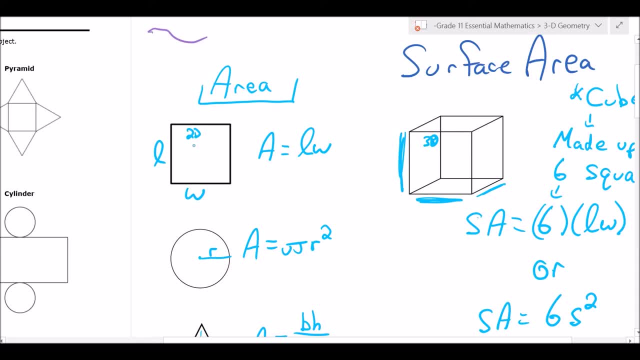 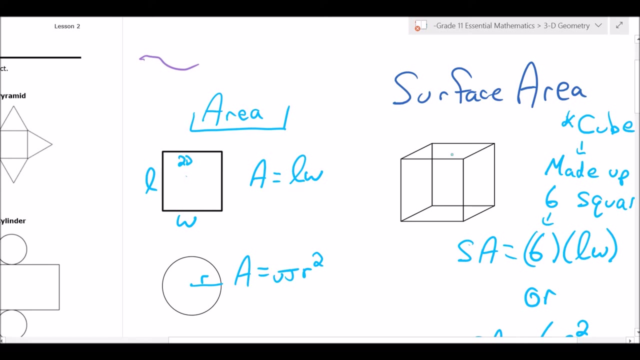 dimension. It's kind of like going from two-dimension when we played Super Nintendo, three-dimensional when we played Nintendo 64, or PlayStation 3.. Now, 3D objects are made up of a bunch of two-dimensional objects, So in this case, if i have a cube, this is called a cube. 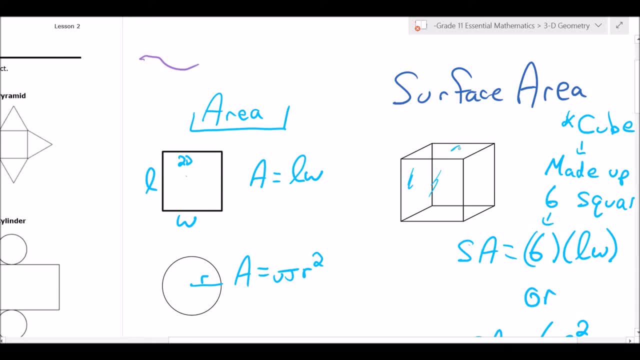 really, what it's made up of is one, two, three, four, five, six squares. Okay, So surface area: i'm looking for the total area of all the two-dimensional objects that are put together to make a three-dimensional object. So let's see if we can cut that down a little bit better. Now let's. 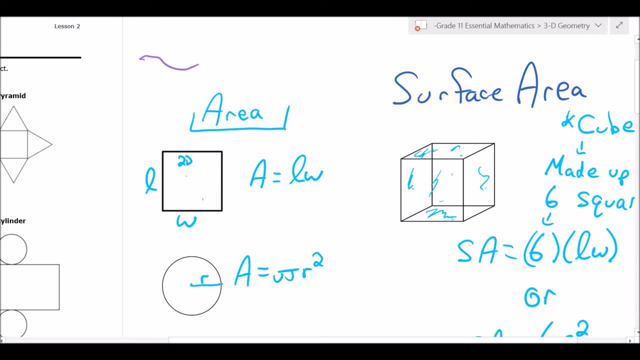 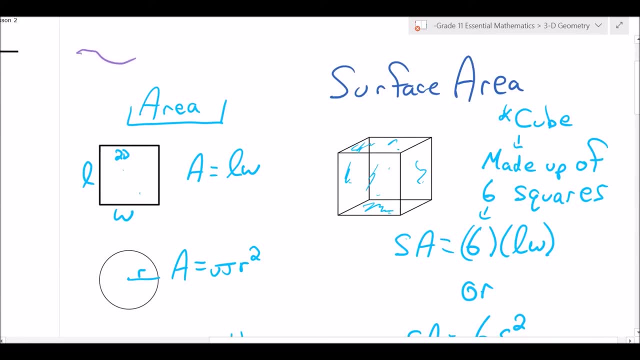 three-dimensional object. So in the case of a cube it's the best example to see. if the area of one square is length times width or side squared, then the surface area of a three-dimensional object called a cube, which is made up of six squares, would be six times length. 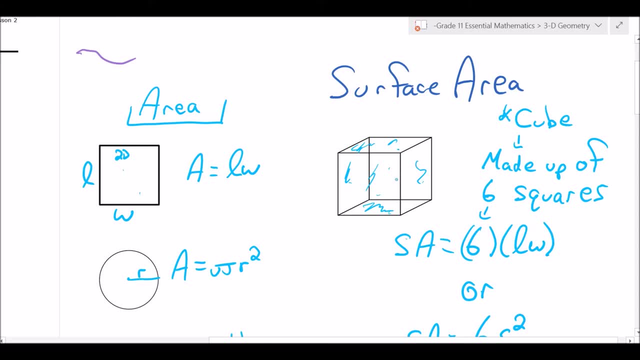 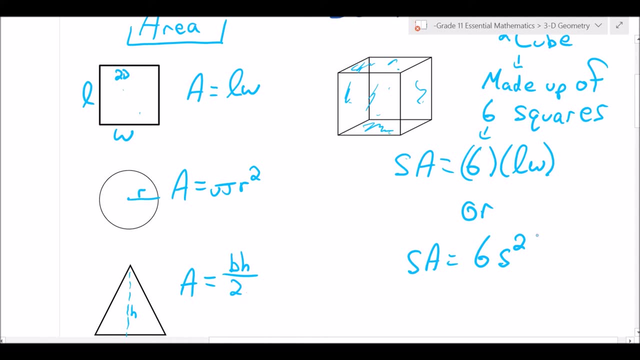 times width, Six squares. the area of six squares added together gets the total surface area of a three-dimensional object. Okay, you can also call it six sides squared, because we know with a cube all of our side lengths will be the exact same size. So length times width is the same as saying: 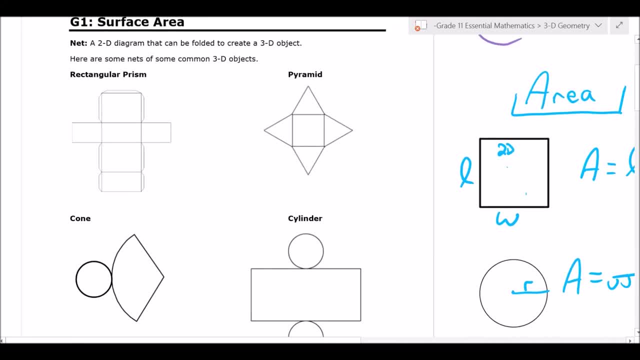 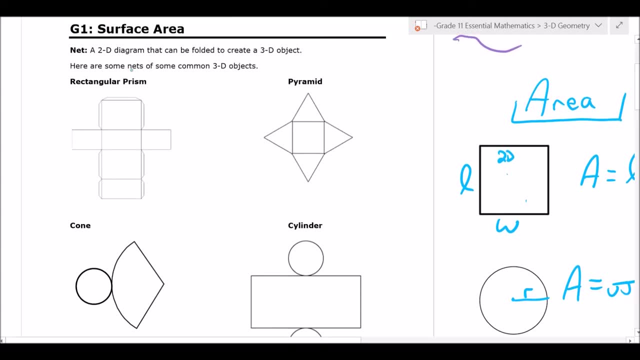 side times size. When we think about 3D objects, like I said before, they're all made up of 2D shapes, So we can break up any 3D object into something called a net. Now a net just shows us. 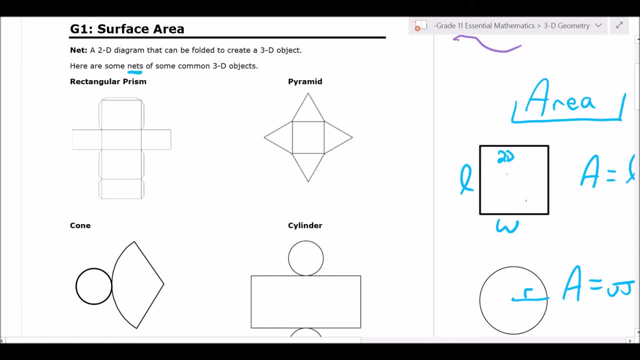 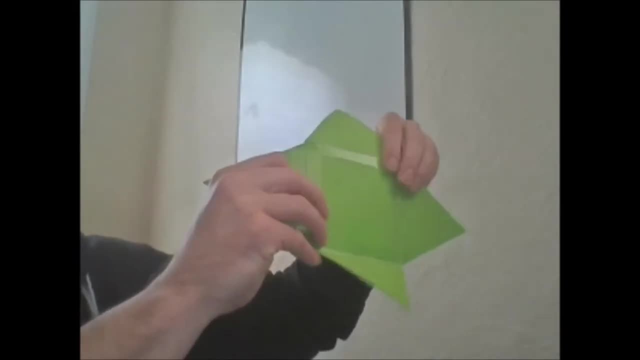 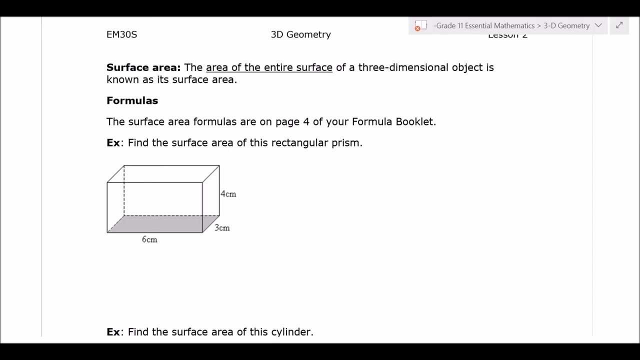 how a 3D object is created by using 2D shapes. Here are a couple of examples that you can see of shapes that I've made, and then I can break them into a two-dimensional net. Okay, the great thing about surface area is really: all we have to do is be able to identify what 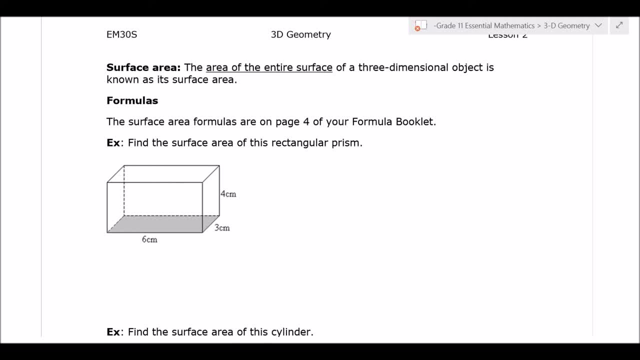 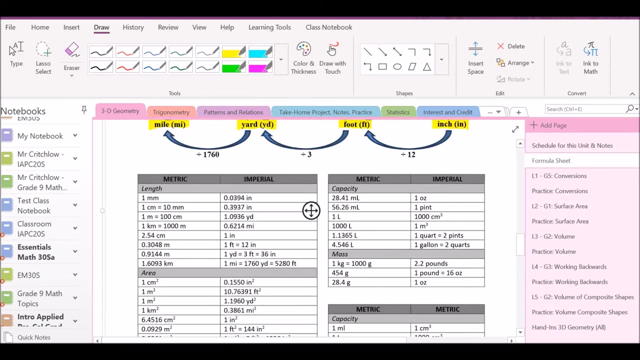 shape we have, identify the dimensions that we need or know, and then identify which formula to use. Okay, so let's look at this first example. We are going to have to use our formula sheet. We're going to look at this chart right up here and we're going to be looking at the surface area. 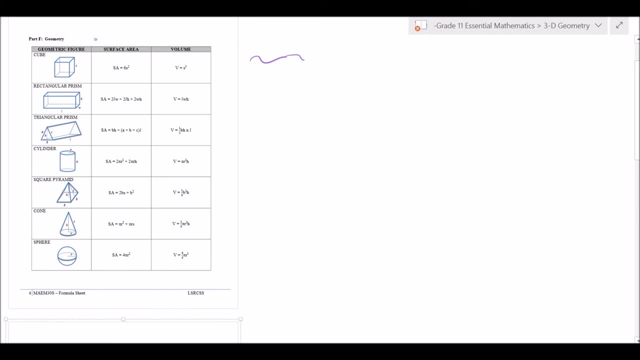 column. So we're looking at this chart: Surface area for each shape is listed in this first column and if we go across the cube, surface area is 65 squared and the rectangular prism is two times length times width, plus two times length times height, plus two times width times height. and we go on and on here with 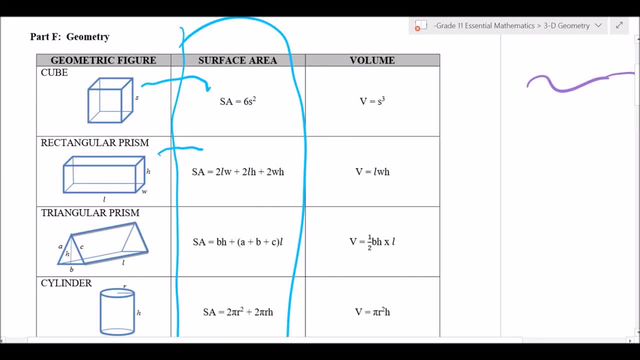 a few more examples. Now what we have to do is we have to look at our shapes, identify the dimensions, the dimensional values, and all we have to do is put the values in for the letter variable. So if I'm looking at a rectangular prism, if I look back to my formula sheet, I'll see that there are three. 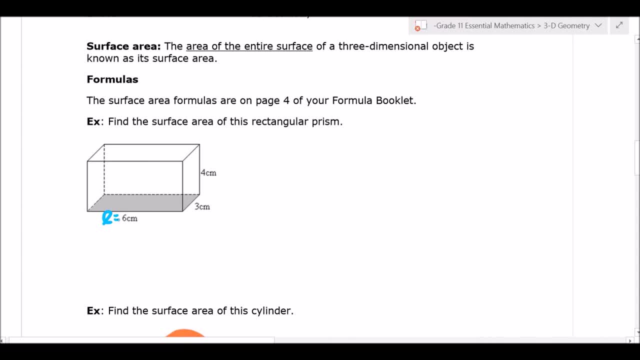 dimensions. I have to label The length, okay. I have to label the width and I have to label the height. So I'm given all three of those dimensions. Now I look at my formula sheet. So my formula sheet tells me I have to. 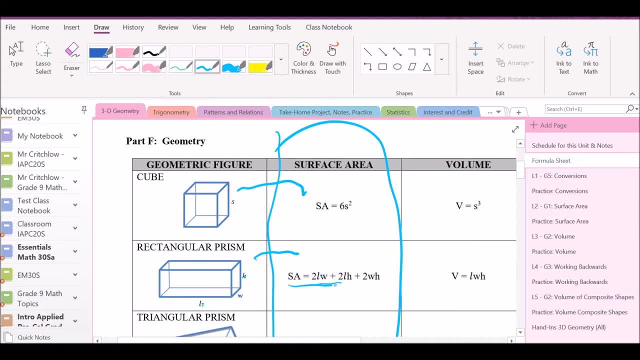 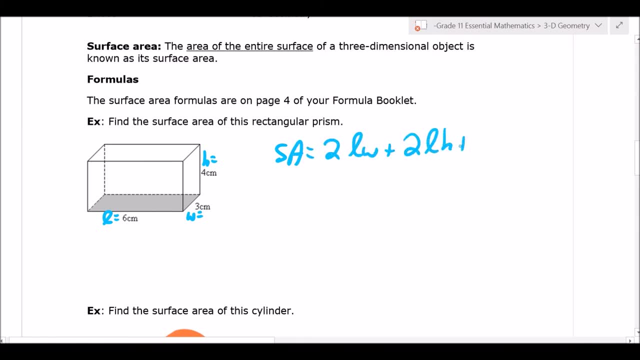 have length, width and height, and then it tells me that my surface area formula looks like this. All I'm going to do is write down my surface area formula. Once I've done that, all I have to do is replace my letter variables. 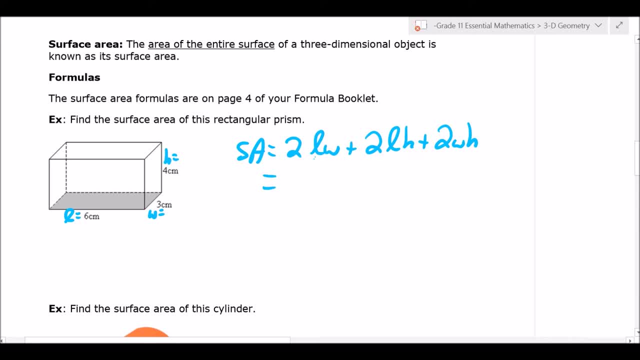 with their values. So I'm going to write down my letter variables and I'm going to write down my value on the shape. So what I mean by that is this says two times length times width, So the two stays here. I put in my length value, which is six, my width value, which is three, plus two times my. 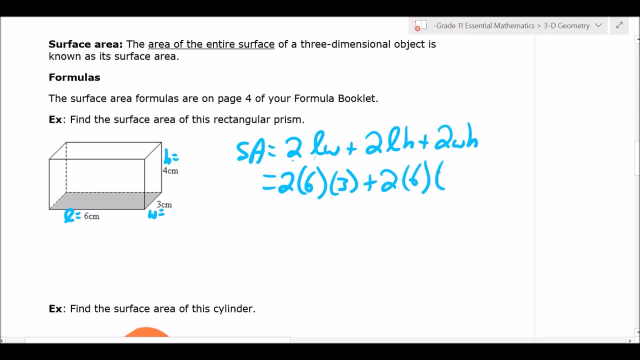 length value, which is six times my height value, which is four, plus two times my width, which is three times my height, which is four. Once I have that set up, all I have to do is put that in my. 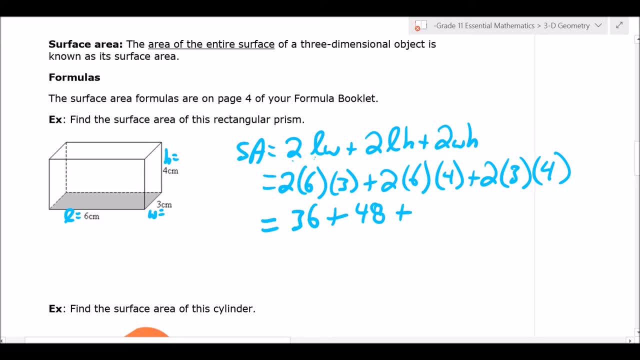 calculator and I'll get a final answer. Okay, so we have 108.. It's centimeters, but anytime we have surface area, surface area is always units squared. The surface area, just like area, is always going to be units squared. 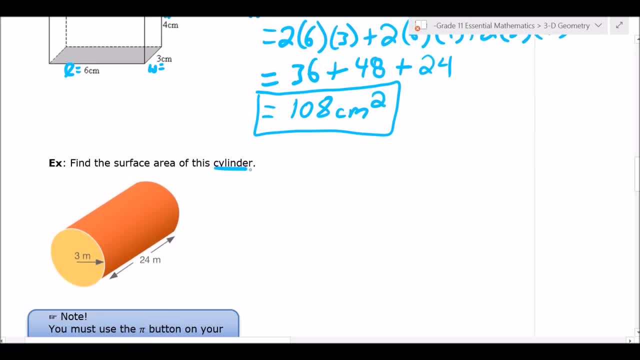 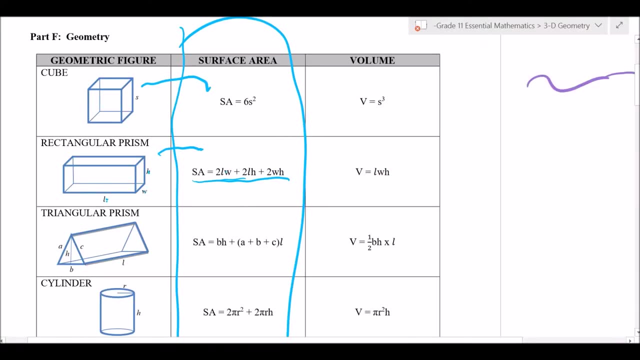 Okay, let's look at the next sheet. So, the shape here is a cylinder. So what I want to do is I want to look at the shape. Okay, this is a cylinder. I go back to my formula sheet. Here's my formula sheet. I look for the cylinder example. Okay, here's a cylinder. 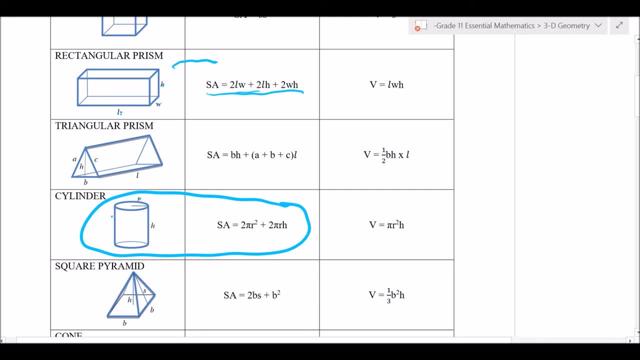 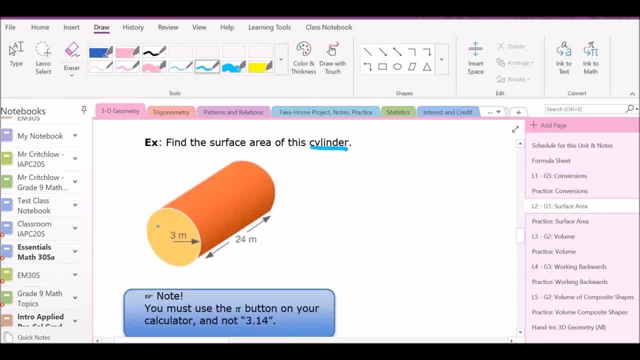 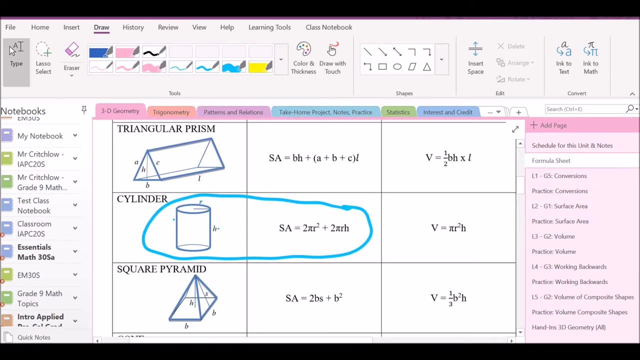 example. And what am I going to have to do? I'm going to have to label the radius and the height. Remember, the radius is half the distance of the diameter. So the radius and the height. Here's the radius, Here's the height. Now I go back to my formula sheet. Okay, here's my formula. 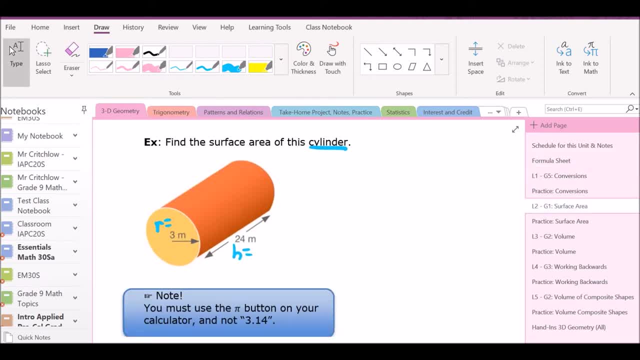 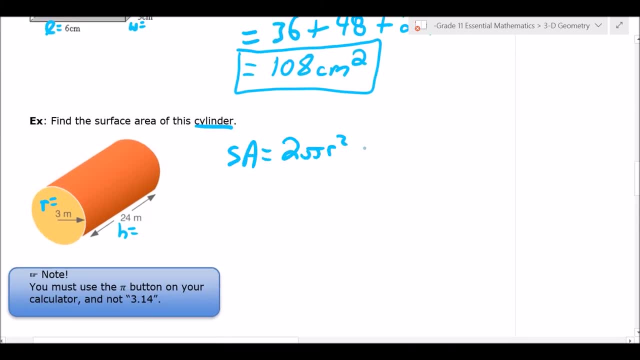 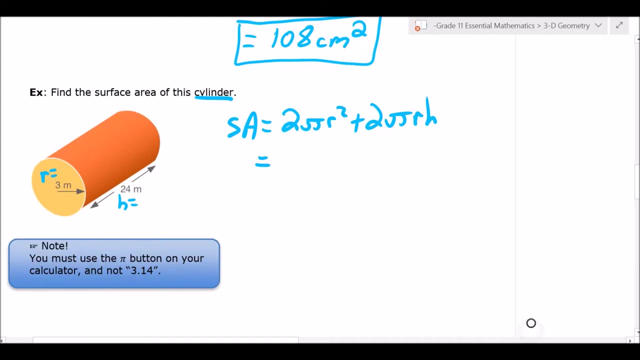 I need to put that into my question to start me off. So I have surface area. but this shape is two pi r squared plus minus two pi r squared, 2 pi r 8.. Now I just replace my letter variables with my number value, So we have 2.. Remember pi. 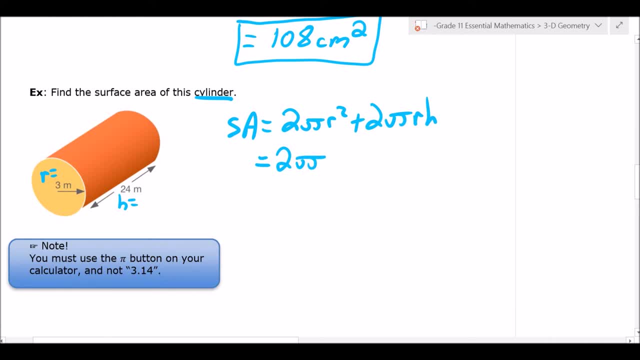 represents 3.14. with continuation of decimal values, r is radius, which is 3.. 2 pi r squared plus 2 times pi, Pi represents a number already. Radius is 3 and height is 20.. If we can put that in our calculator, we'll get a final answer. The final answer is 508. 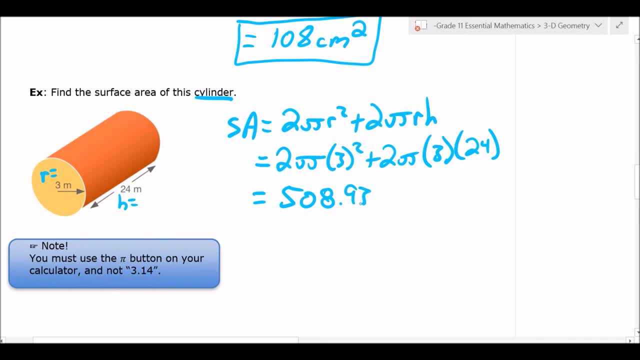 decimal 938.. We want to round to two decimal places, So we're going to round up because this guy is larger than 5.. So it's 508 decimal 9 for meters. Remember, for surface area it's always units squared. Okay, one important thing to remember: we want to use the pi button on our 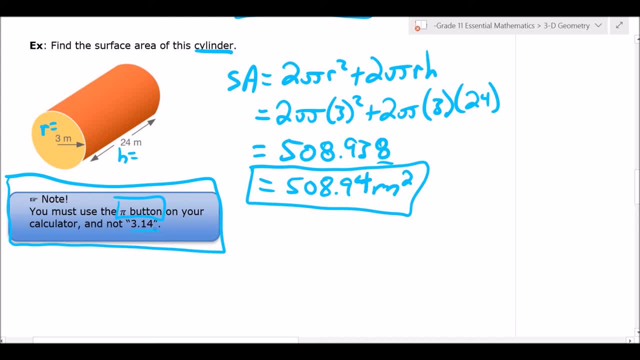 calculator to get the answer. So we're going to use the pi button on our calculator to get the answer. So we're going to use the pi button on our calculator to get the answer. So we're going to calculator: We use 3.14.. It's not as accurate because we actually have a few more numbers. 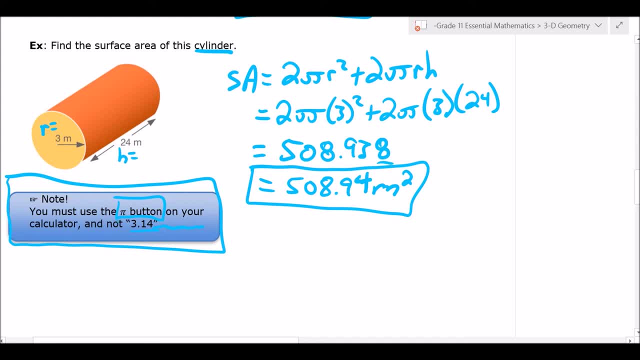 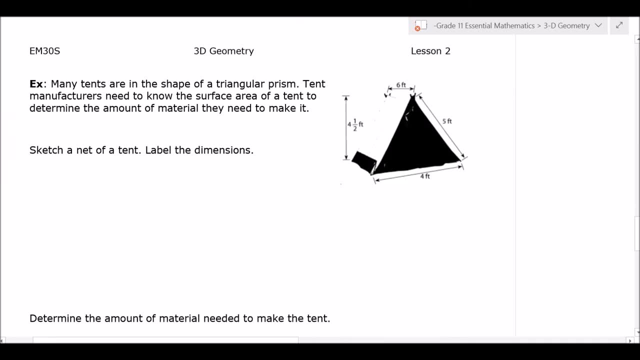 as decimals as this coupon. So use the pie button. That's an exact value. Don't use 3.14 for this question. Okay, one more example. This one has a couple aspects to it. We have a triangular prism. Okay, so we know the shape. They want to know the surface area of the tent, because if they know the 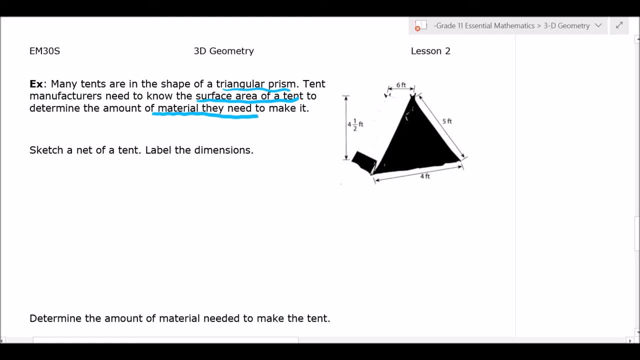 surface area of the tent. they'll know how much material they need to make that. The first thing it says is: can we sketch a net- This is a two-dimensional net- of a tent- and label the dimensions? So basically what it's saying is it wants us to draw this shape. 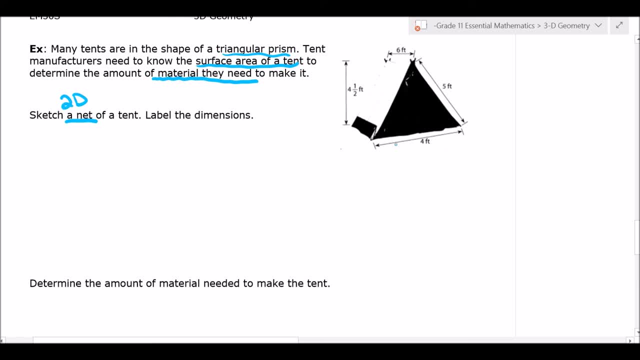 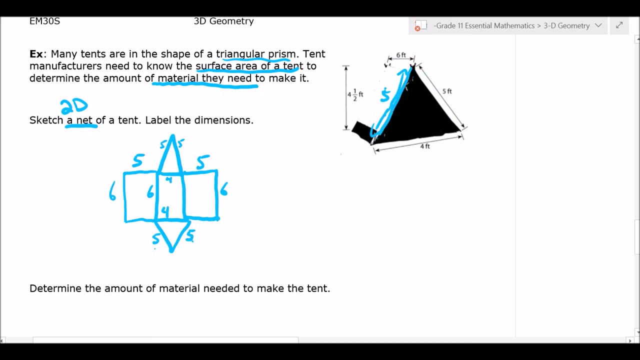 broken up into its two-dimensional parts. So let's do that. We can see that the bottom here would be rectangular side rectangular, side rectangular. and then we have a triangle on the front and back. Okay, now let's just look at what this shape looks like. So we have a two-dimensional 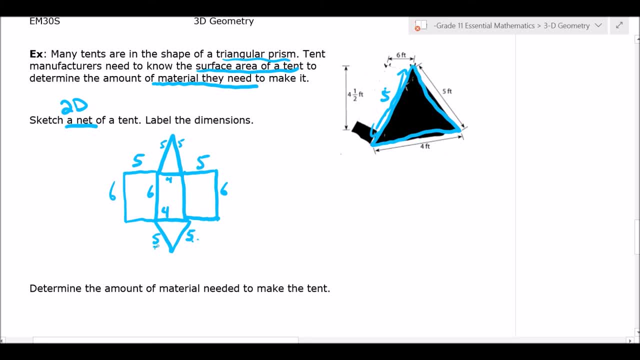 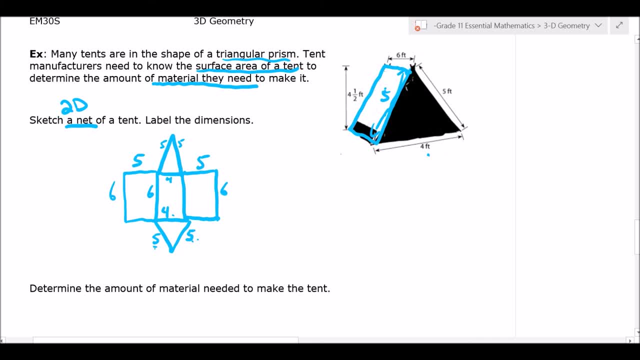 perspective there that shows us a rectangle. The height is five feet, okay, and the width is six feet. We got that right. If you look along the bottom here we're going to have a rectangle along the base Just going to draw it through the shape, that triangular prism- Okay, the one length. 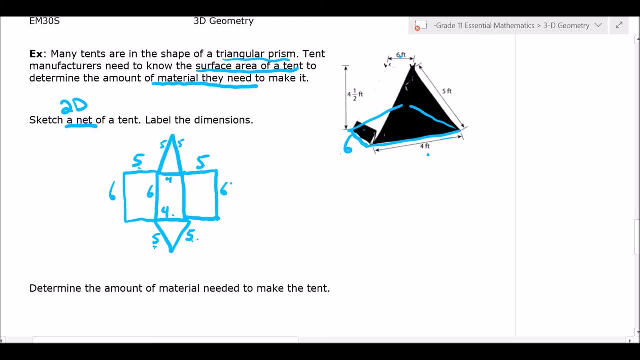 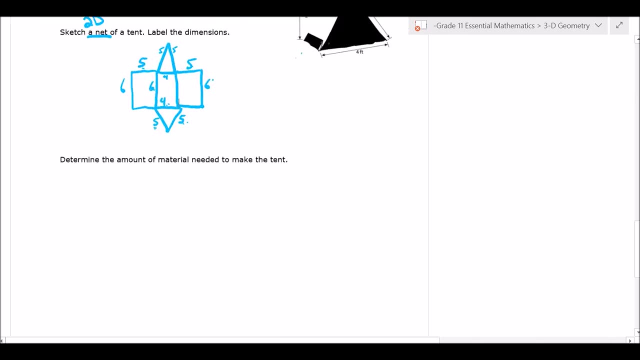 is four feet, Good. And then the side length we know is six feet, because it's the same as up there. So we have four by six, And now we've found all the shapes that are two-dimensional that make up our 3D object. Okay, the next step is that we want to look at the amount of material needed to make. 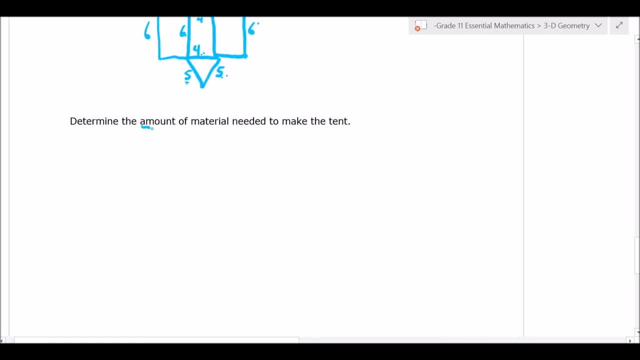 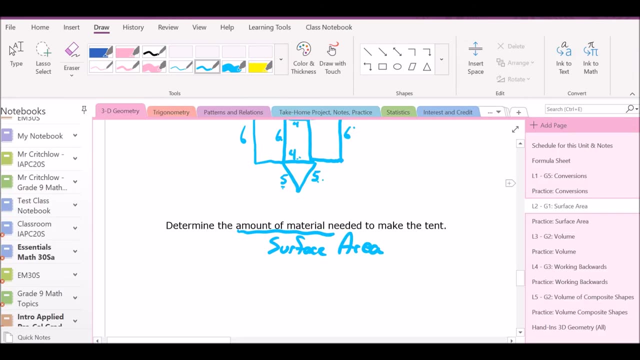 the tent. So we want to look at. we'll ask: how much material do we need? That is a surface area question. We look back to our formula sheet. We're going to look at the amount of material needed to make the tent. Oh, formula sheet's, here We're looking for a triangular prism. Common mistake is: 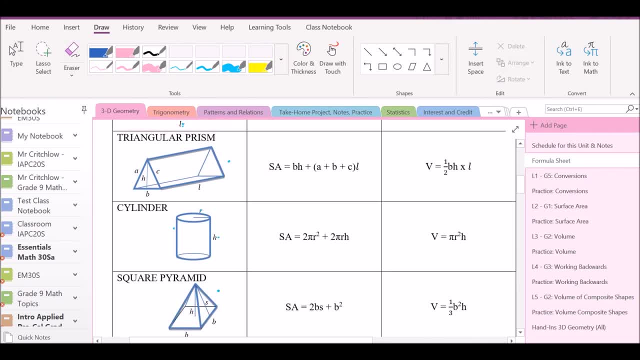 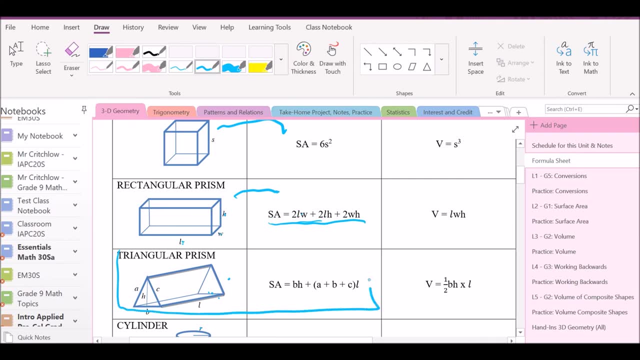 that we get triangular prism and square pyramid mistaken for each other. Make sure you guys are identifying the right shape, In this case the triangular prism. what we're looking for: we want to label all of these values on our triangular prism and then we're going to use 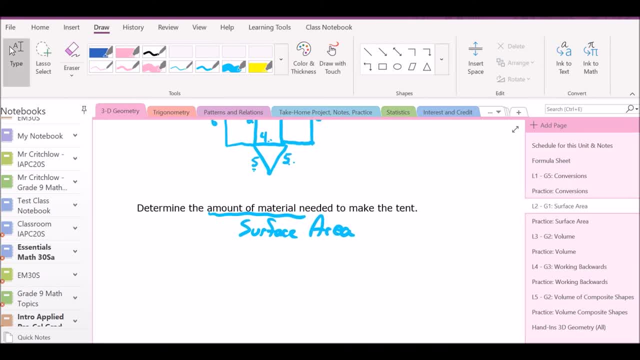 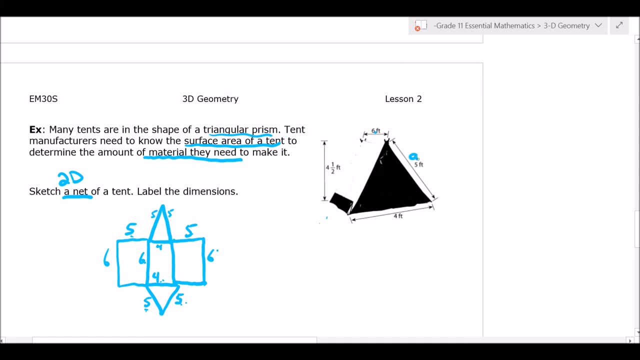 this formula. We'll go back to our question. Go up here. You guys will have your formula sheet inside you. We're going to reference that to label. So five will be my A value. If that side's five feet, this side is also five feet and that's going to be my C value: Four feet along the bottom. 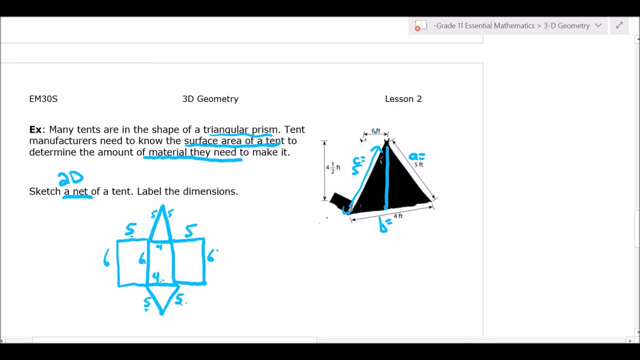 is my B value, my base. My height from here to here is actually given on the side here. So the height is equal to four and a half feet, And then we'll have one more value. We need to know our length. Our length is six feet. 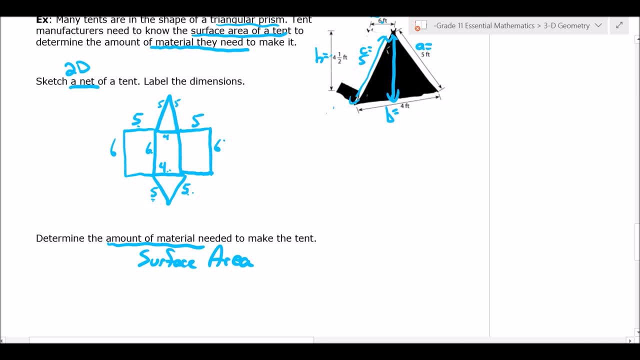 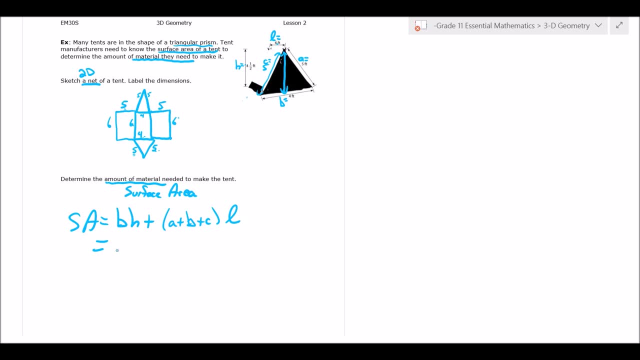 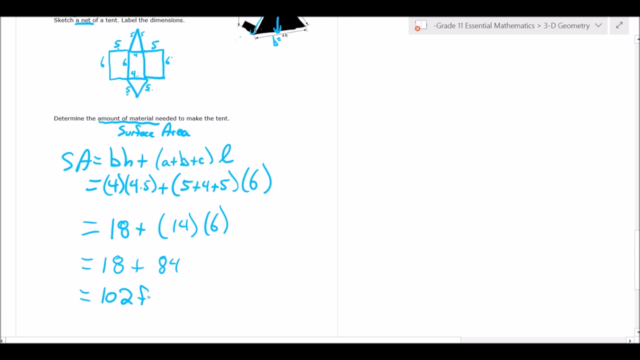 We've labeled all the values shown on our formula sheet. Now we write down our formula. That's the next step. We have 102 feet. Remember, units are squared surface area. Okay, There's a few more shapes to work within our lesson and hand in, but this is the basic idea: Identify the dimension. 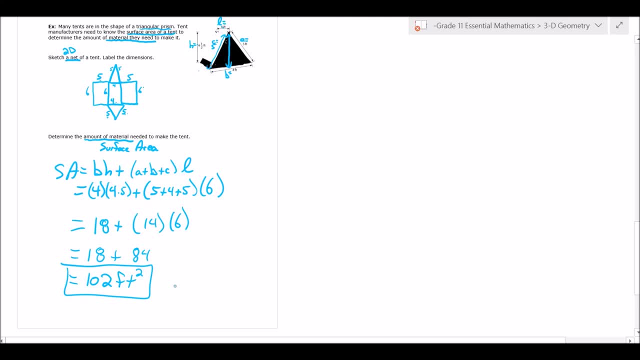 write out our formula, fill in the values for the formula and just put it in your calculator and get your answer. You don't have to show these steps. I just did that because I was doing mental math. You can go straight from this step for a final answer using a calculator. Okay, Have a. good day and I will talk to you guys next week.